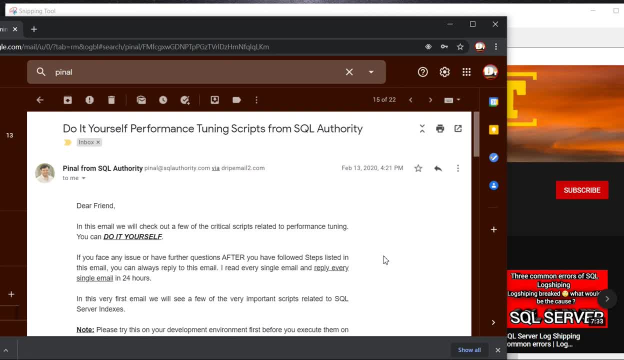 the session. I would like to say thanks to Pinal because I got something from directly from the Pinal side and which helps a lot. I use this. you know steps to improve the performance and I really shocked when I use these steps to you know improving the performance and it was really helpful. So I'm going to tell you how we can do. I directly. 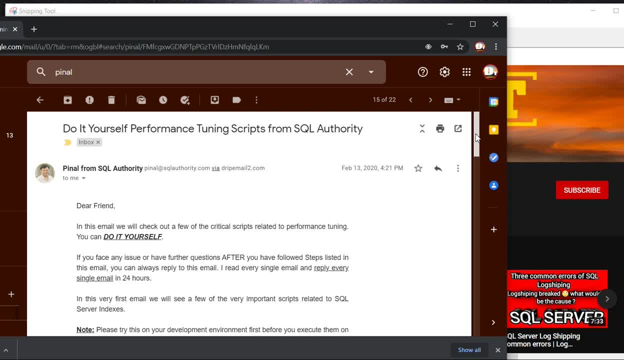 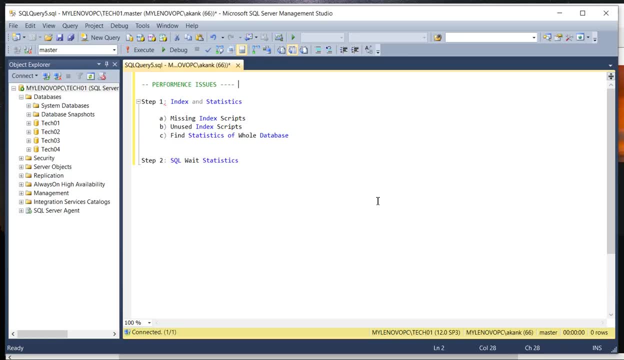 got it from the, you know, the Pinal side SQL authority, So I really thanks to him. okay, So just now I need to connect my SQL Server Management Studio. okay, So if you are looking, the performance issues, these three, two steps and these three, four parameters which you need to start as soon as possible. Once you start this, you know, troubleshoot your performance definitely will improve. 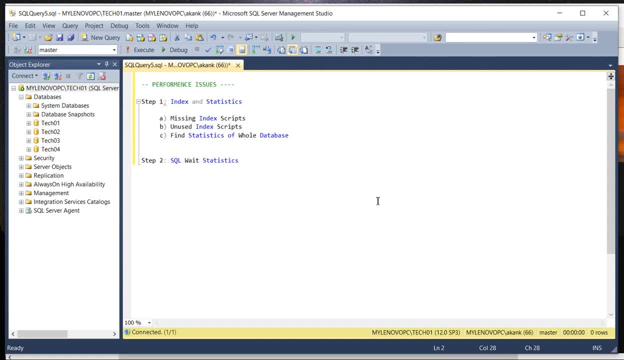 As soon as definitely it will improve the. you know so here if you see the steps one, index and statics. So I have mentioned the three things which you need to check under the index and statics. The first is missing index script. The second unused index and third is static of the whole database. okay, And in 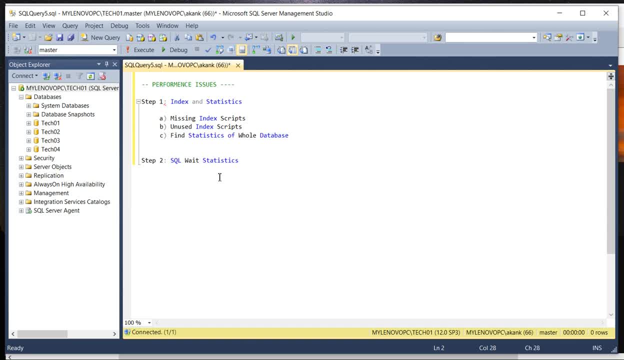 Step 2, you need to check the weight statics. So I am going to tell you how we can do which script is helping here. If you need a script, I will give the script. you just do a comment, I will share with you. 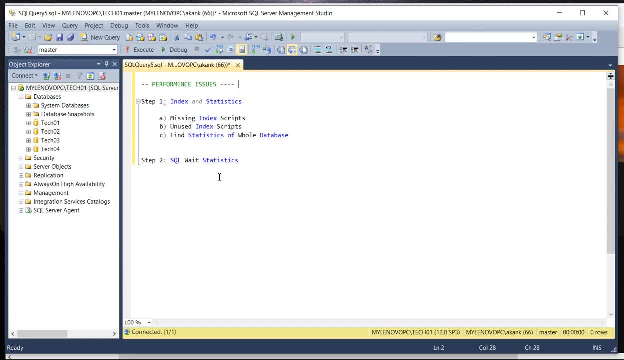 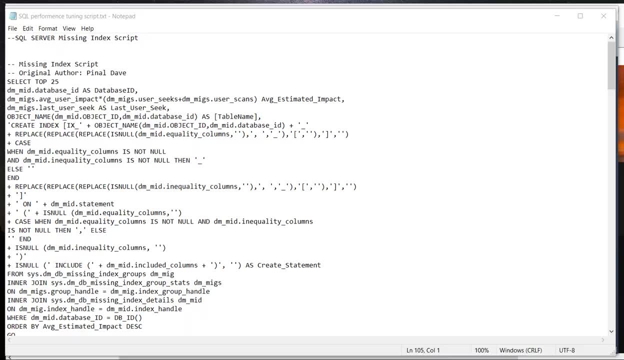 and you also try it. definitely it will improve your performance As soon as you start these things. definitely it will improve. So I am going to just you know, opening my script. So first you need to identify the missing index script. okay, 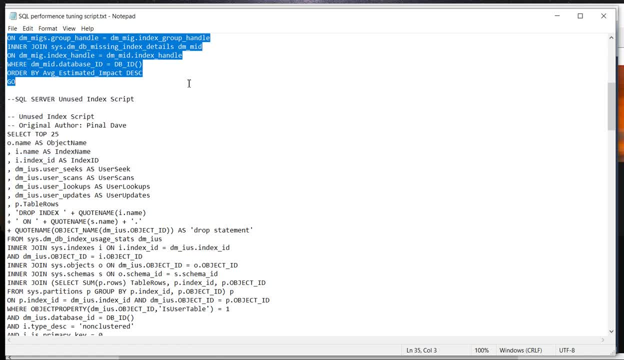 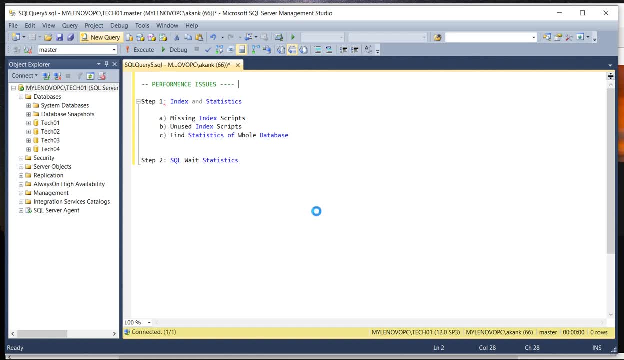 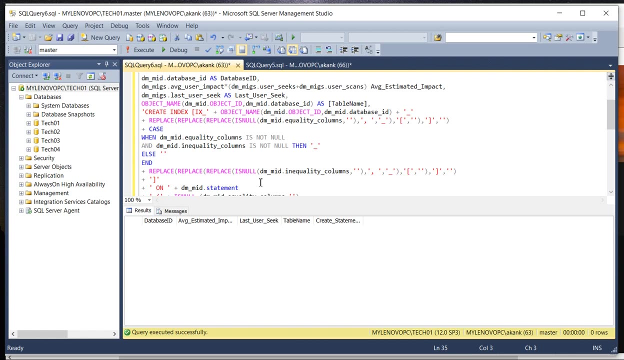 So let me take the script from here and I am going to execute right away and we will see whether it is helpful or not. okay, So this, the first step is you need to identify the missing index. So basically it is saying if index is really missing. 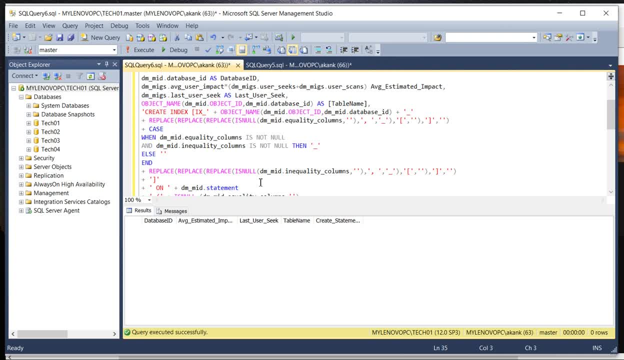 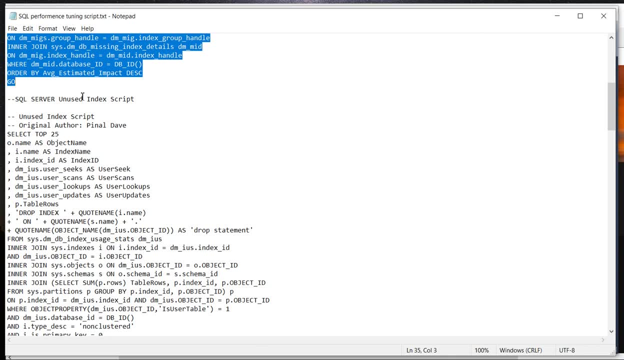 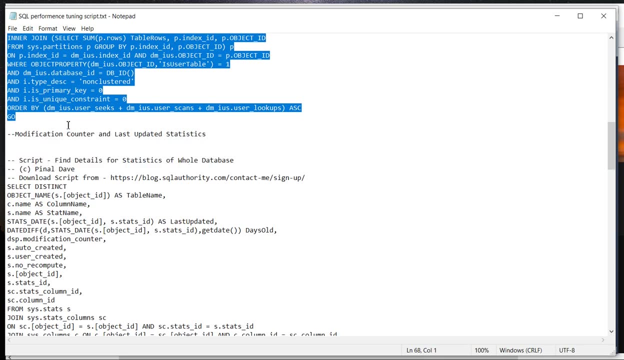 If index is really missing, which causing the performance, then definitely you need to trigger those index and you need to create the, you know missing index. The second is the unused index. This is very, very helpful. N number of times we didn't focus at all and we simply created the index, but we are. 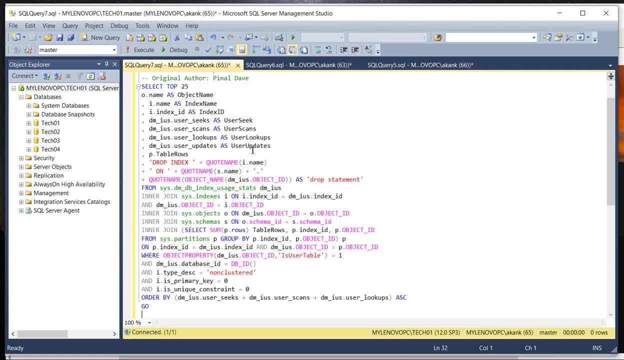 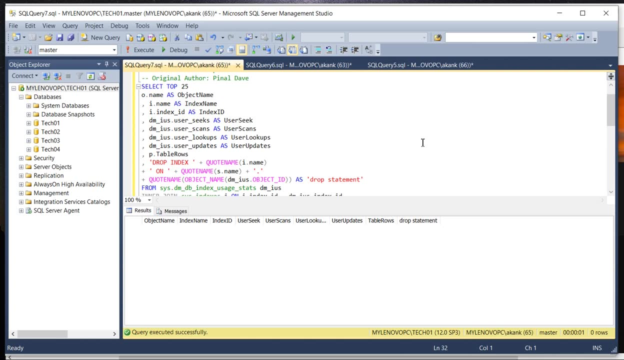 not aware whether that index is useful or not. whether the index is, you know regularly it is used or not. right, That is really causing the performance improvement. So once you find the unused index, definitely you drop it. actually, If the index is not used in couple of months or years you should drop that index because 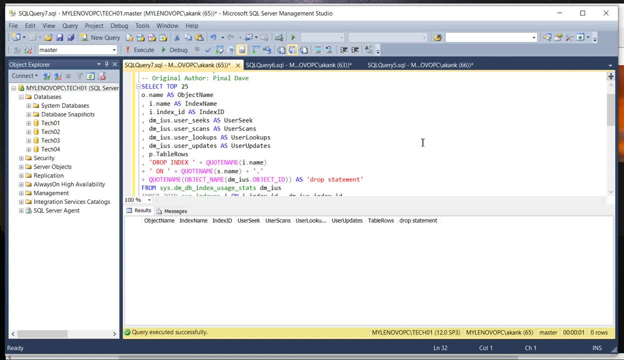 definitely unused index will cause 100% performance issues. okay, We several times we didn't focus at all. These are the small, small steps but we didn't check the regularly right. So unused index, 100% causing the performance issues. 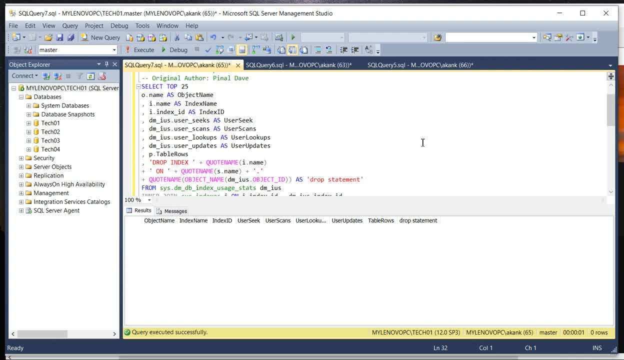 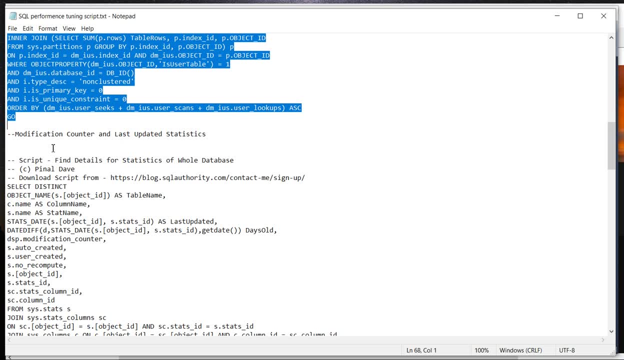 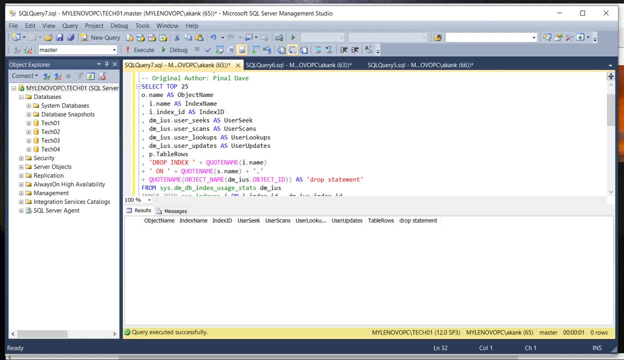 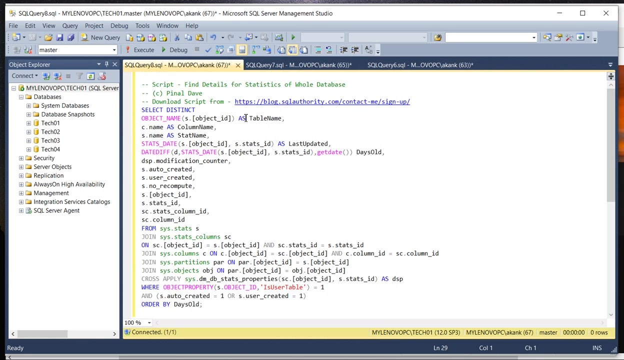 That is really helpful. if you, as soon as possible, you drop the unused index, definitely your performance will improve. The third: the modification counter, the update static. as we all aware, our statics should be updated. Okay, If your stats is not updated 100%, definitely it will cause. you know the issues for the 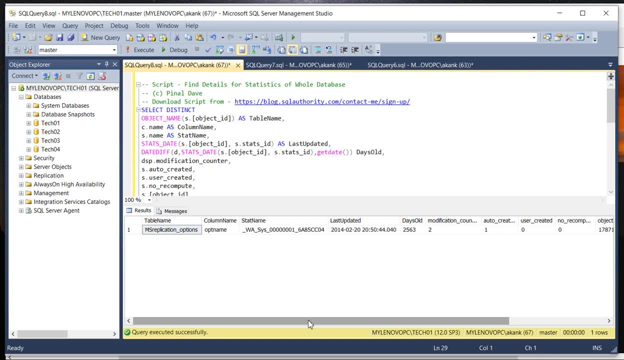 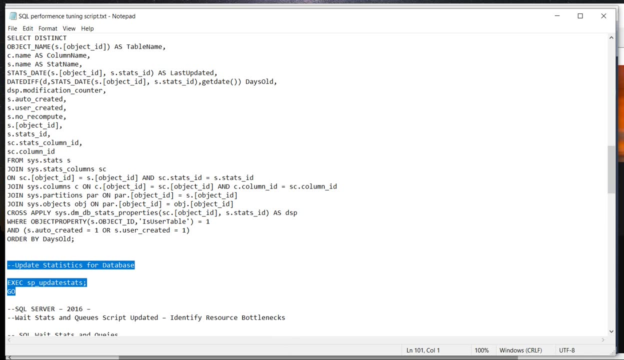 performance. So, as you can see here, it will give you the complete details about the statics, whether updated or not. You can use this script, okay, and you can update stat if you, if you want to do the update stat. 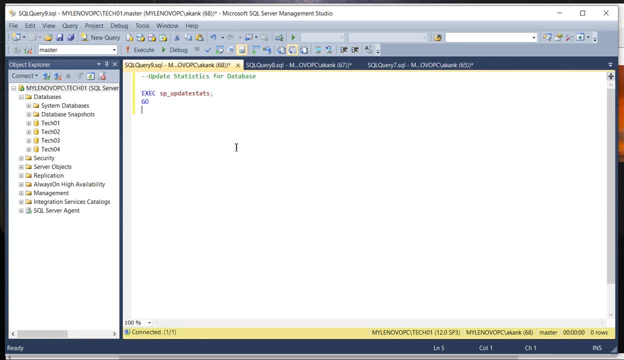 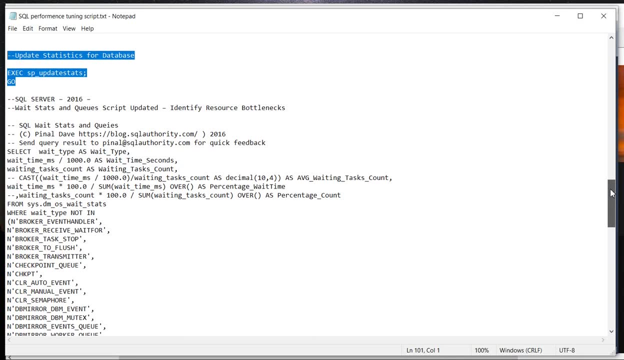 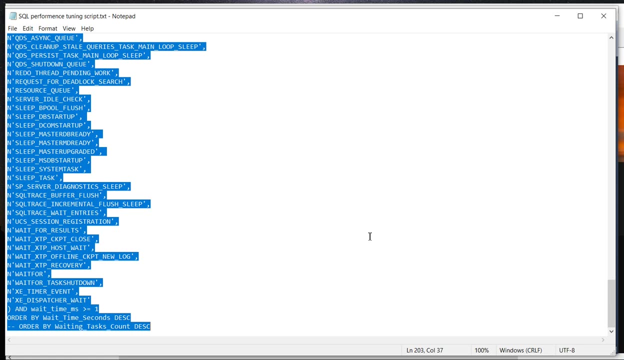 You can simply execute the update stat, as we all aware, the SP command. we can use the update stat. The step two, which is really helpful for SQL Server 16, I'm going to tell you: for SQL 16, you know, we need to identify the percentage of, you know, the wait time. 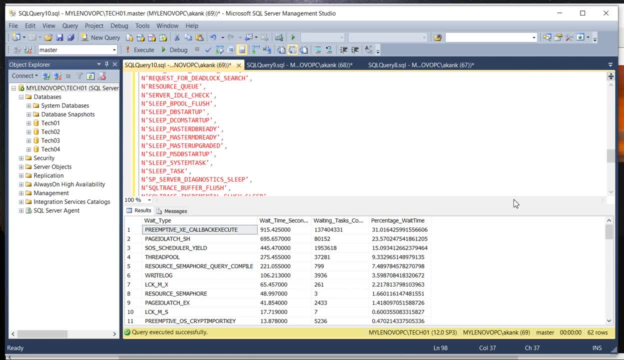 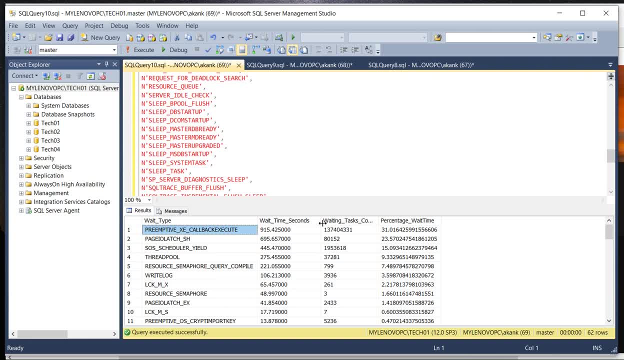 The wait, the type of wait and the wait time is really correlating the performance issues. You need to identify the wait type. which type of wait is causing the problem. That's really helpful to improve the performance as soon as you identify the wait type. the 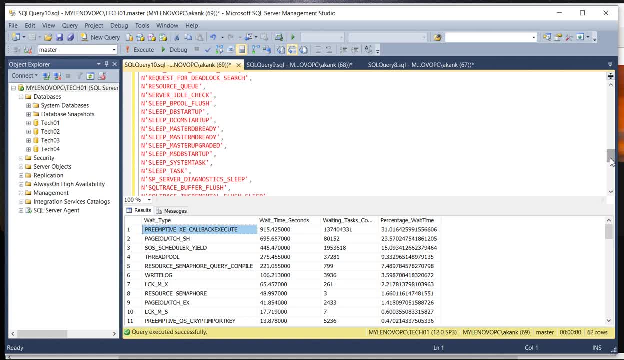 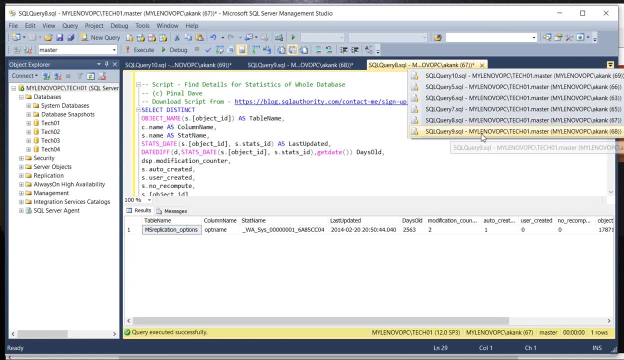 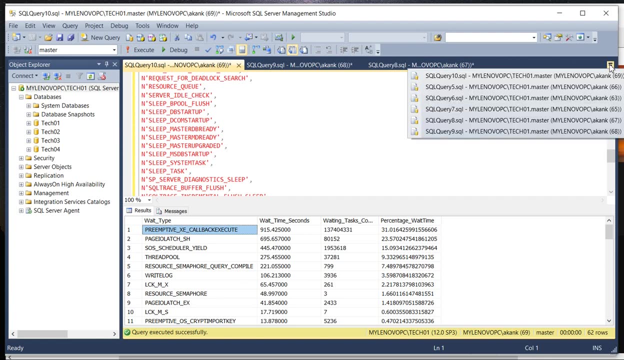 you know your solution will be shorter. It will resolve the issue as soon as possible. So these three, four component the checks. basically you need to check very regularly. As I said, as soon as possible you can drop the duplicate index. 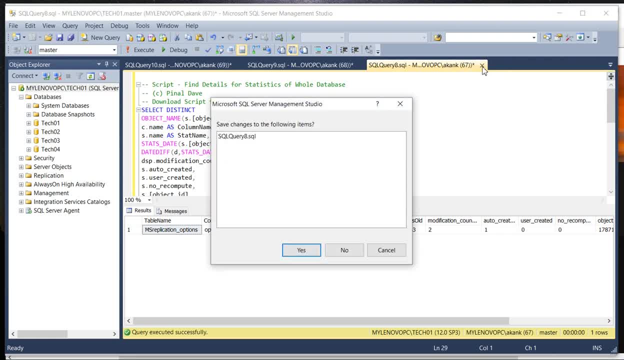 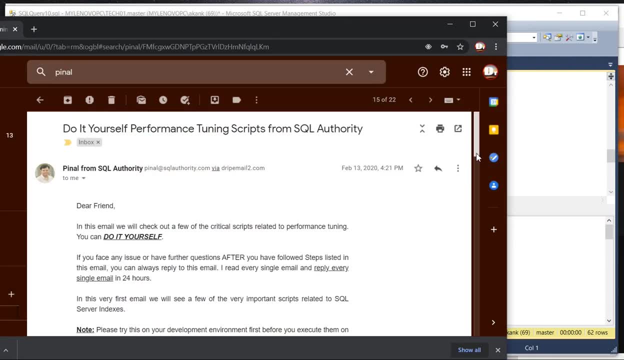 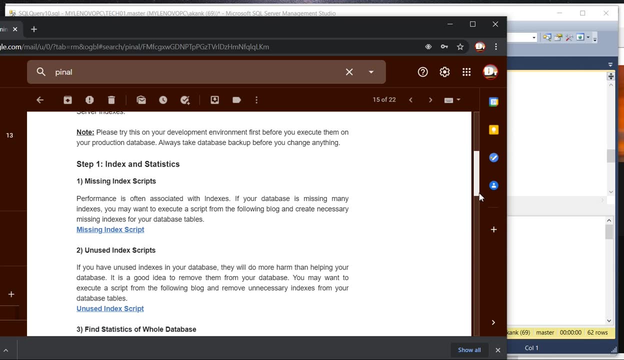 You will get the, you know, the performance improvement. your performance will be improved. So what I'm referring here, I'm not doing anything, I'm just simply referring the penal statement. okay, So these three, four steps which really help help your, you know, to do the performance. 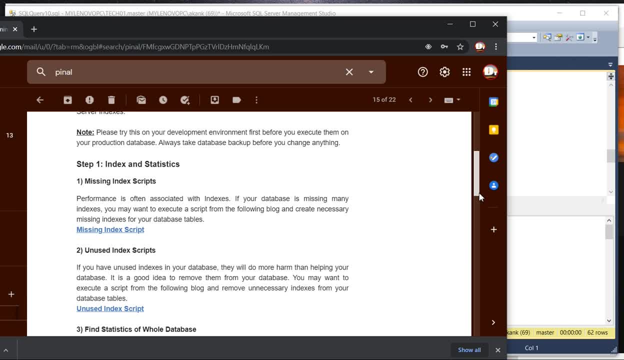 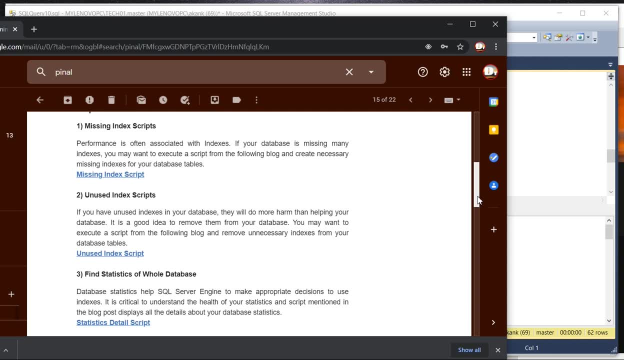 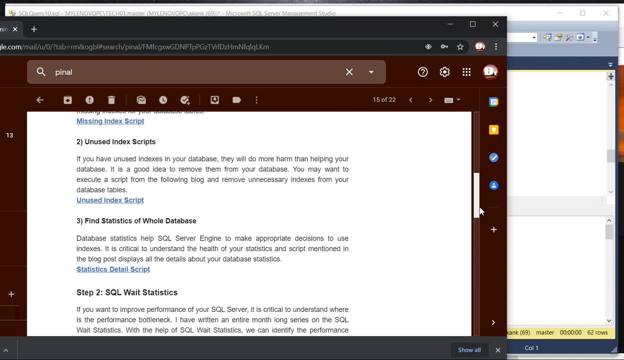 analysis. So, basically, the missing index unused, you know index, and the stat static. Your static should be, you know, updated. It will really help to improve the performance. So that's it, guys, for today. 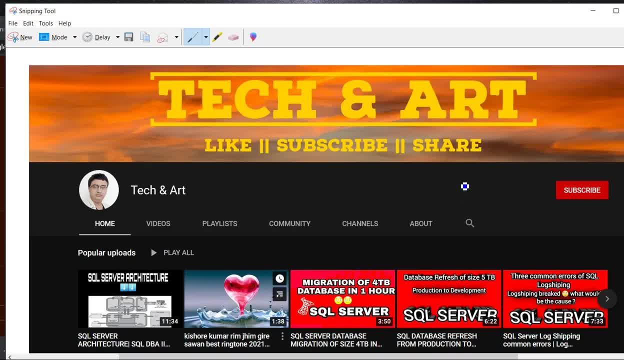 If you need the script, you do the comment. I will share with you. I will email you, okay, And you can also use while doing the performance issues queries. okay, It will really help you Till then. thanks for watching. 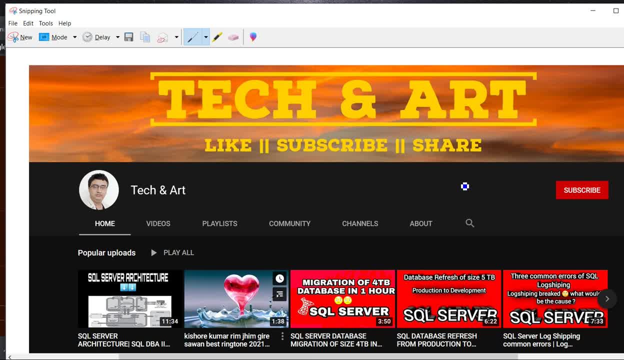